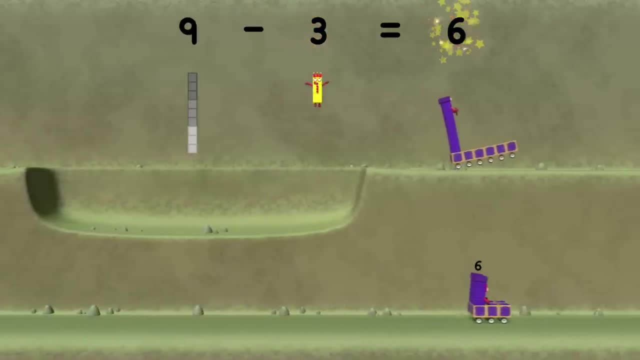 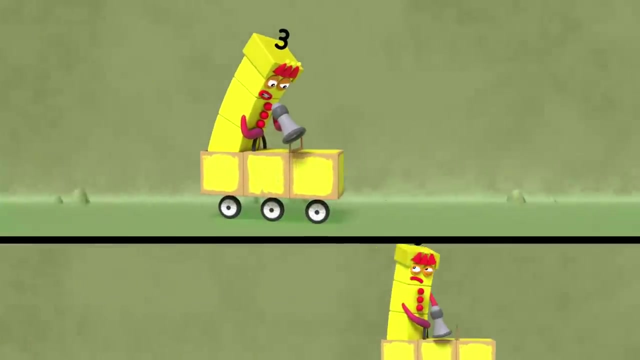 9 minus 3 equals 6.. And the double dipper is in Double dips. six minus three equals three. And what a cloche for a nine. Six couldn't get fine there, Do you mind? I'm commentating here. 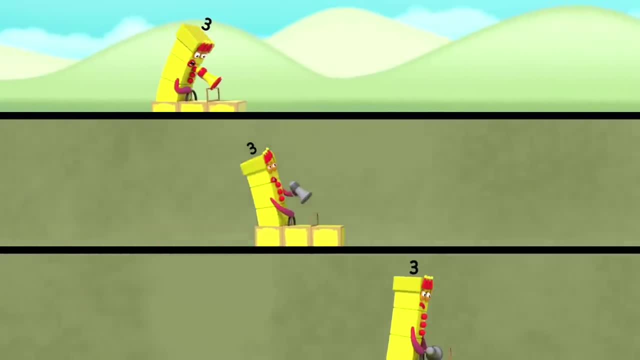 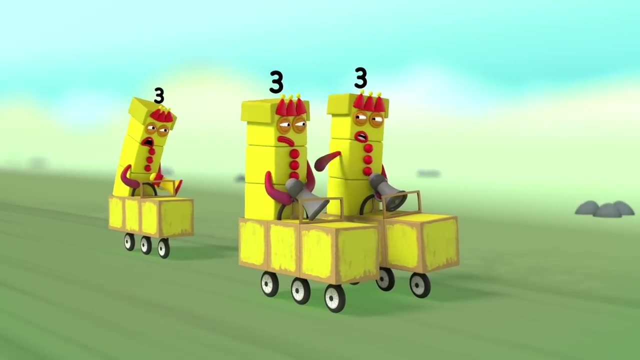 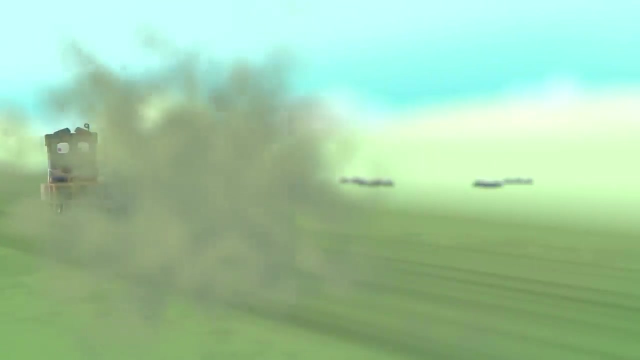 No, I'm commentating, No, I am Me, me, me, Me, me, me, No, me, me, me. Yeah, pull yourselves together. Three plus three equals me Back in action And with the finish line in sight. 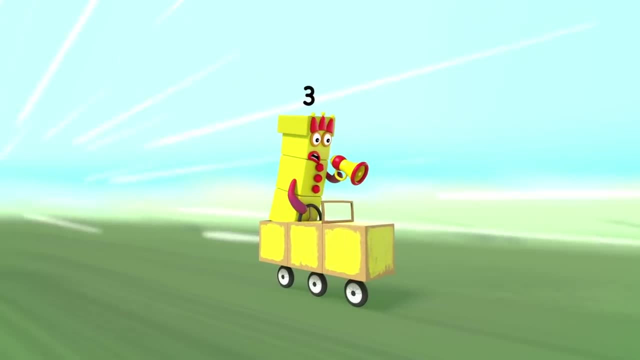 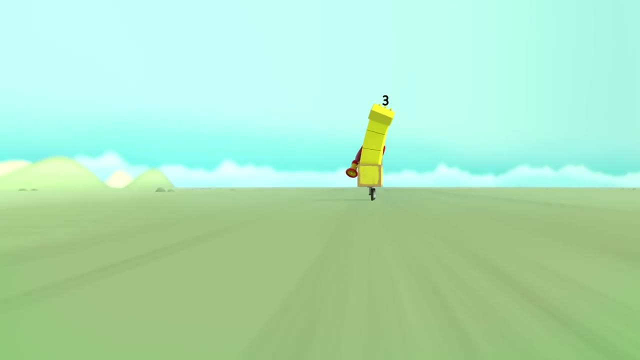 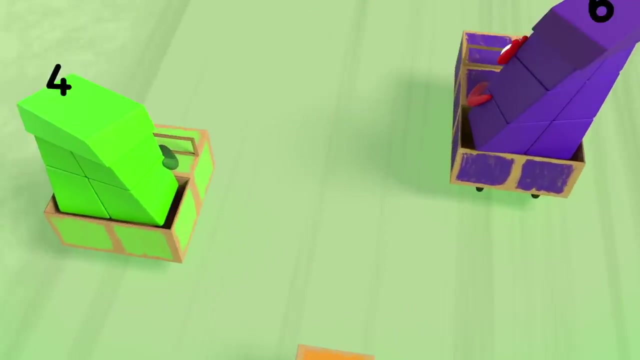 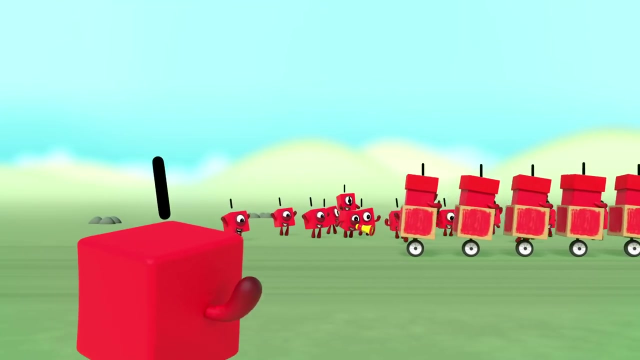 it's four in the lead, then I need a breather Octoblock coming through. Uh-oh, uh-oh, uh-oh. And it's one in the lead, followed by one, but here's one coming up on the inside. 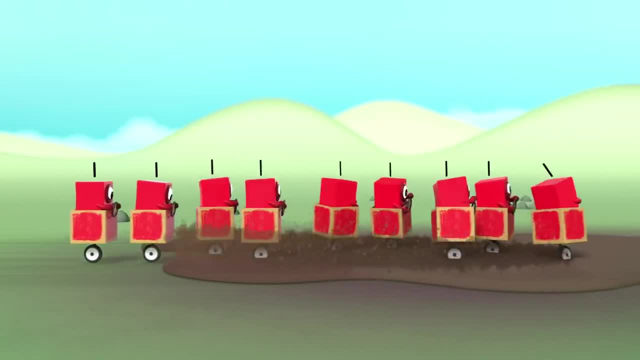 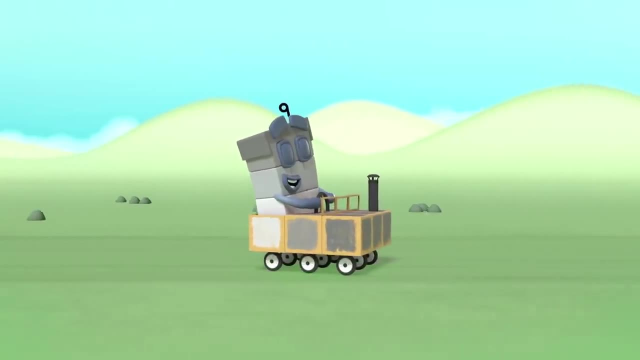 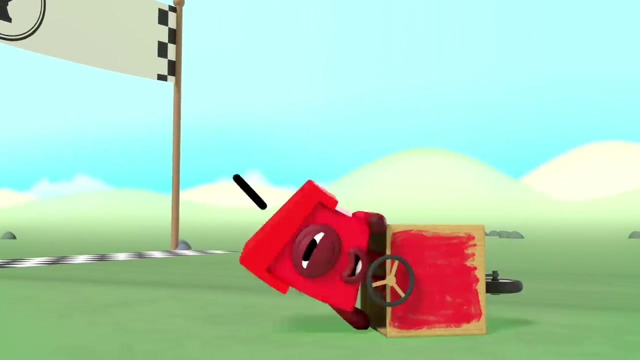 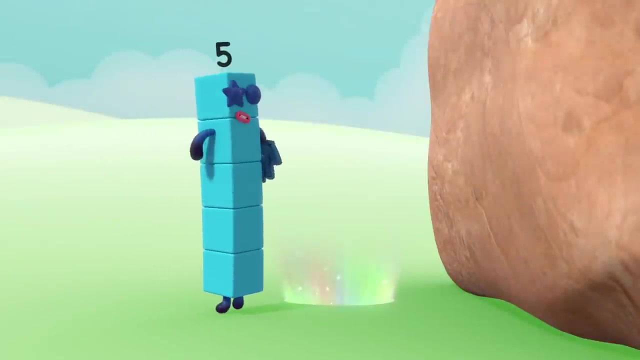 Nine wolves equals Nine. Nice day for it, I'm first. Oh yeah, What is that silly sound? Is that silly sucking sound? Oh, look a hole so big and wide. Why is it there? I do not know. 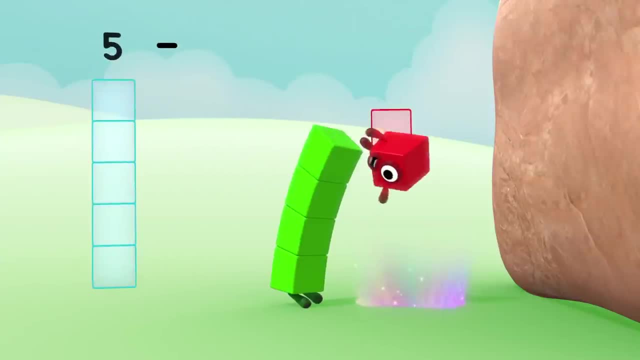 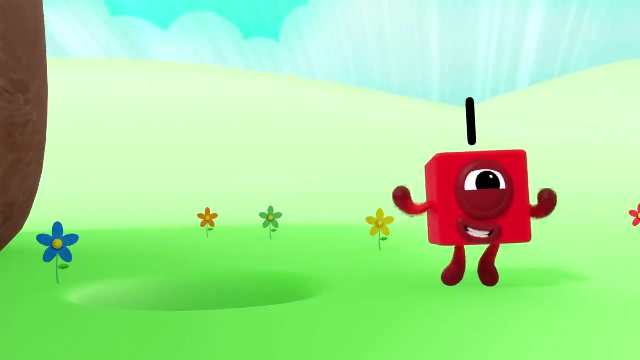 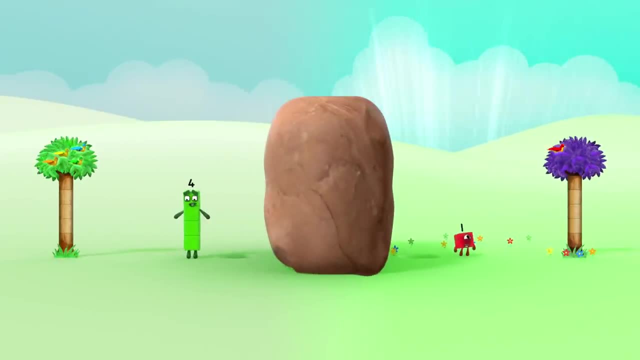 Now, I am four, and here I am. I am one, Here I am. What a wonderful day to be alive. What a wonderful day to be alive. But where, oh, where, oh, where is Five? Five is gone. 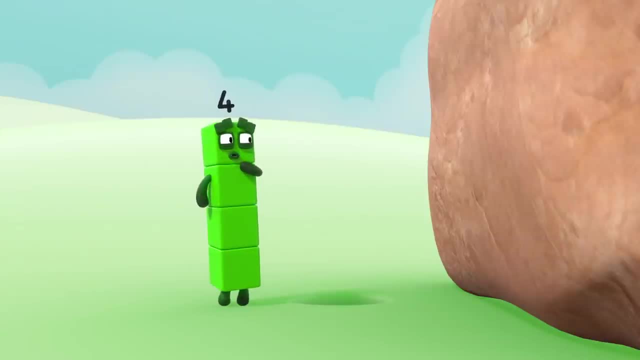 Where did she go? Is she all right? I do not know. Is she here? Is she there? I must keep looking everywhere. What is that silly sucking sound? A giant hole so big and round? Why is it there? I do not know. 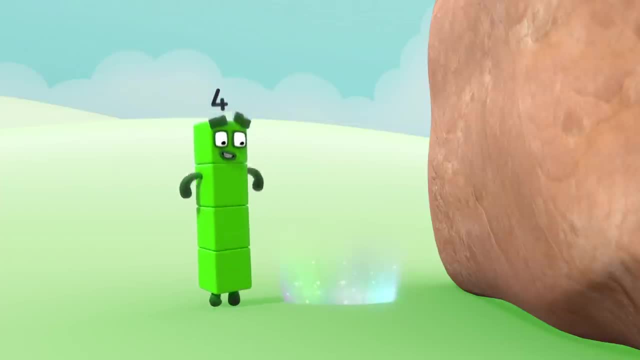 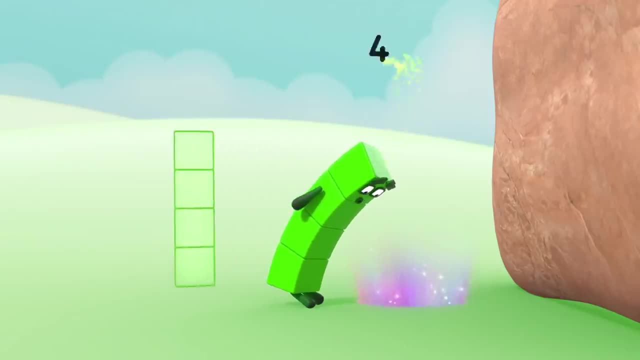 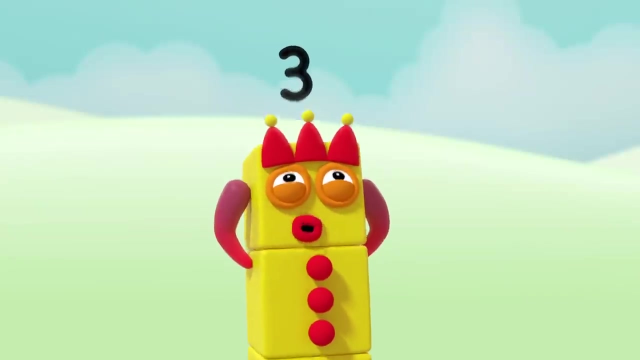 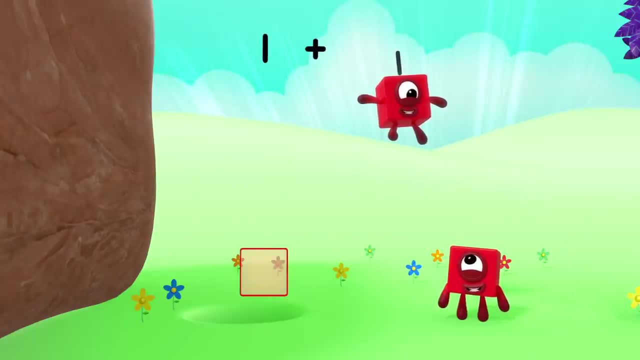 One plus one equals two. What is happening to me? I just got bigger, Did you see? Now I am three and here I am. Now I am two and here I am. What a wonderful day to be alive, I do not know. 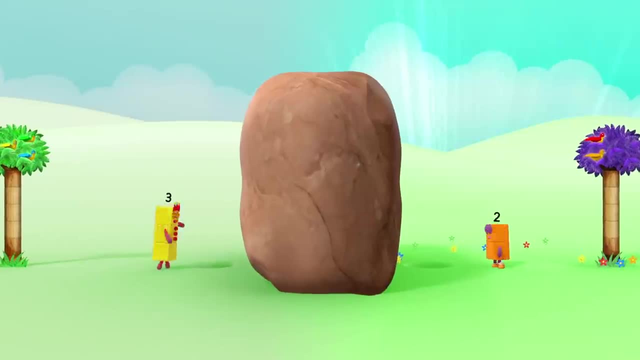 What a wonderful day to be alive. I do not know. I wonder what is down below. Where, oh, where, oh, where, oh, no Alive, but where, oh, where, oh, where is five? I was five, then four, then three. 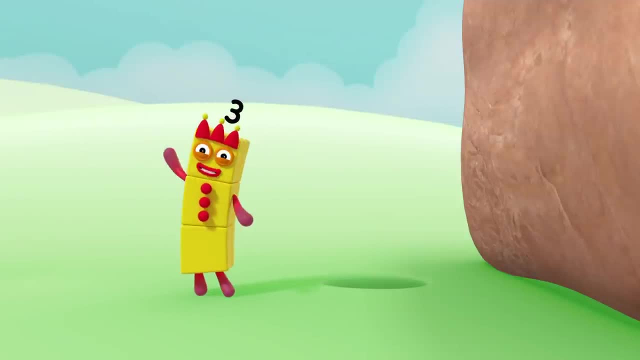 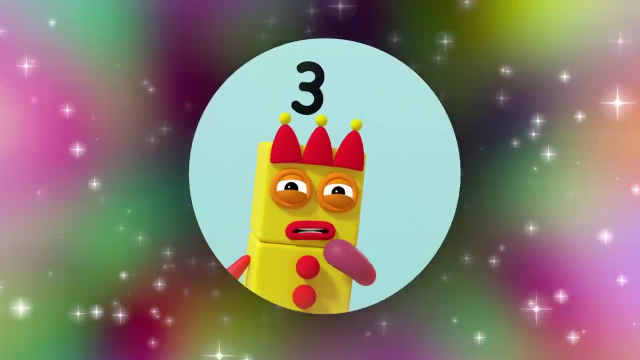 Someone has played a trick on me. I do not mind at all. you see, Three is who I want to be. What is that silly sucking sound? A giant hole so big and round. Why is it there? I do not know. 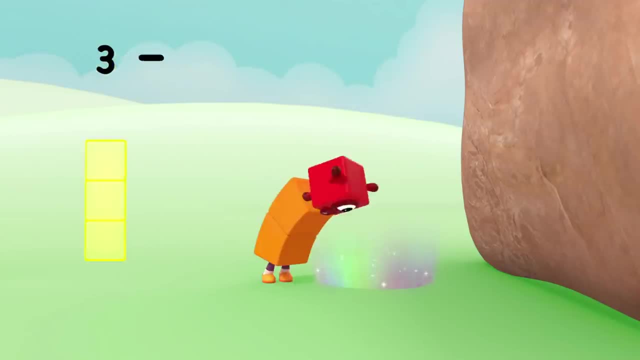 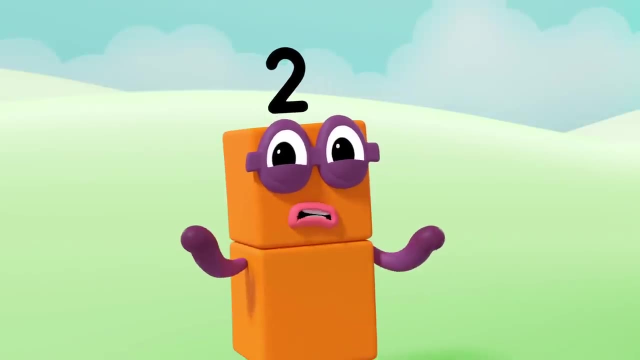 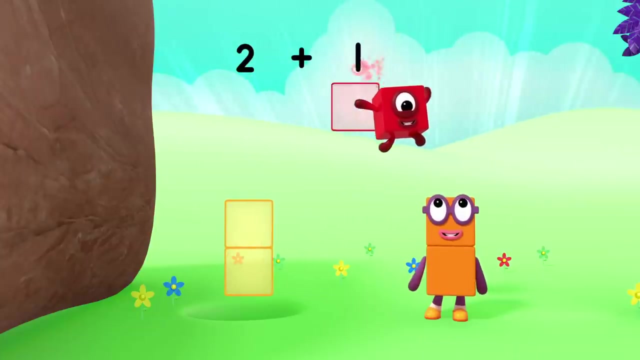 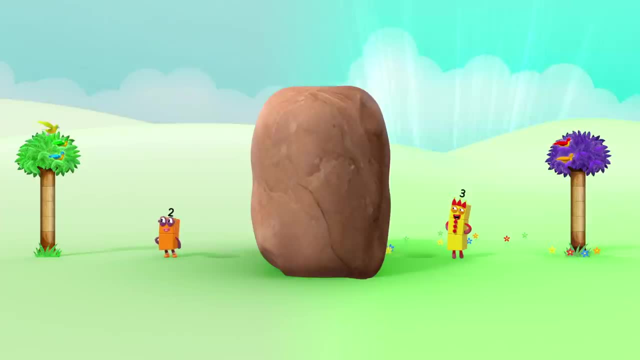 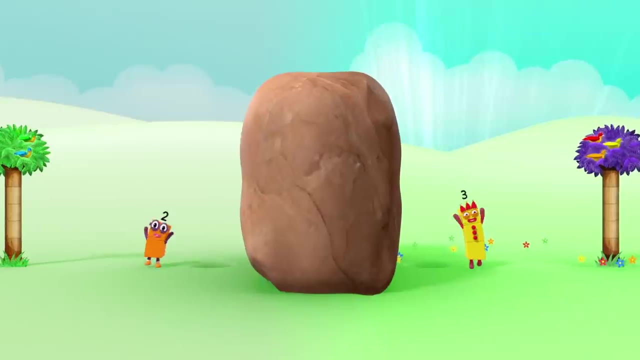 What is happening to me? I just got bigger, Did you see? Now I am two and here I am. Now I am three and here I am. What a wonderful day to be alive. but where, oh, where, oh, where is five? 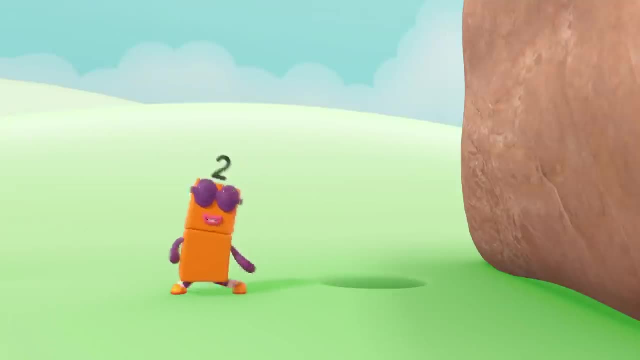 I wonder where the ones will go. I think I've got it Now. I know Every time we get one smaller, somewhere else is getting taller. What is that silly sucking sound? A giant hole so big and round? Why is it there? I do not know. 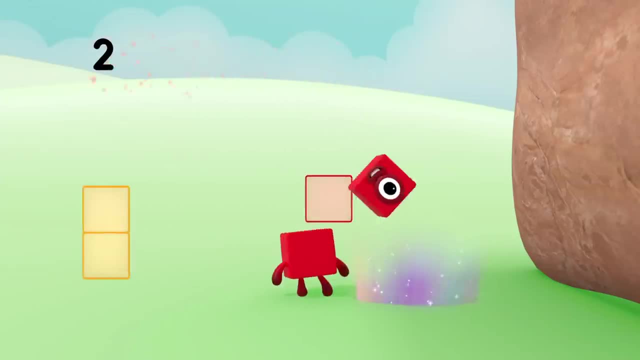 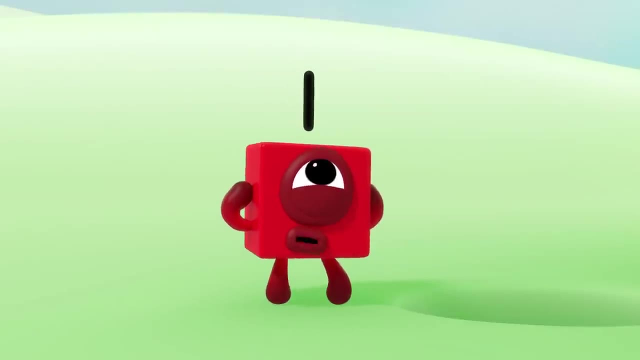 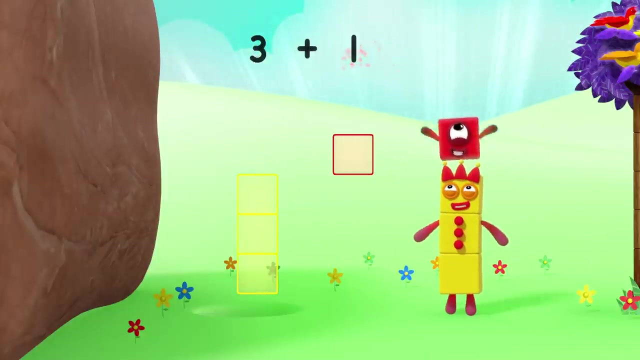 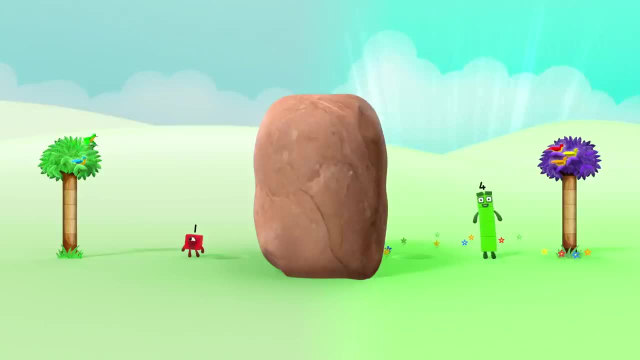 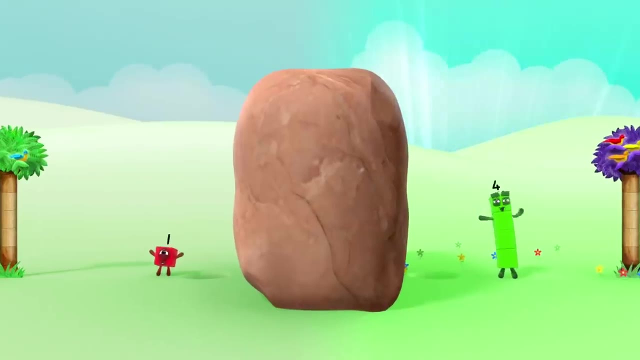 What is happening to me? I just got bigger, Did you see? Now I am one and here I am. Now I am four and here I am. What a wonderful day to be alive. but where, oh, where, oh, where is five? 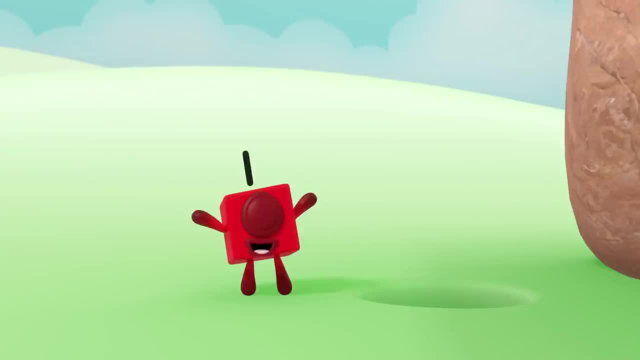 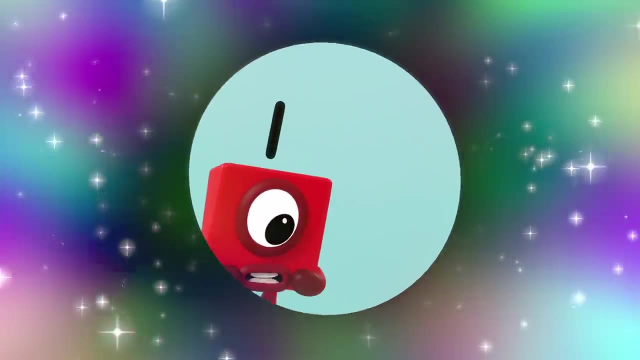 Five, four, three, two, one. Someone's having lots of fun. Now I know where five will be. Four is waiting there for me. What is that silly sucking sound? A giant hole so big and round. Why is it there? I think I know. 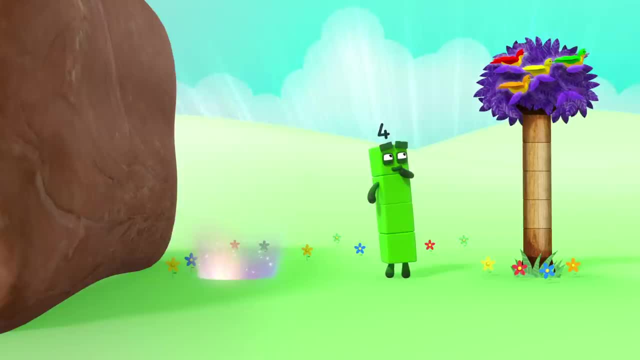 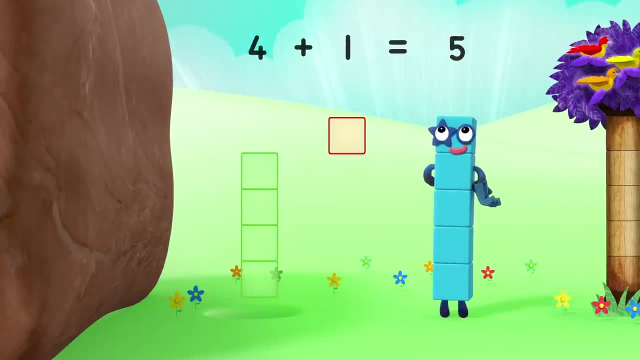 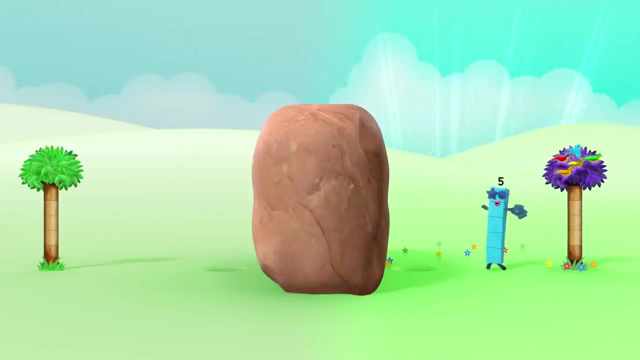 I think I know what's down below. I am one. That was fun. Four, Three plus one equals five. What is happening to me? I just got bigger. Did you see? What a wonderful day to be alive. but where, oh, where, oh, where is five? 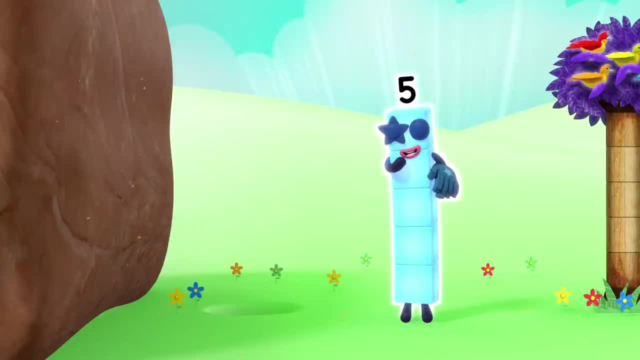 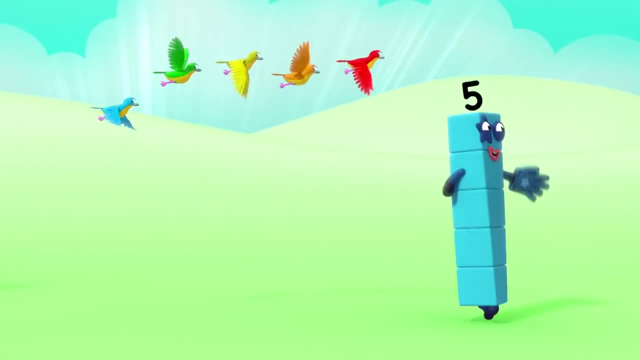 Here I am and I am five. What a wonderful way to arrive. One, two, three, four, five. What a brilliant, amazing, fantastic, terrific and wonderful day to be alive: One, two, three, four, five. 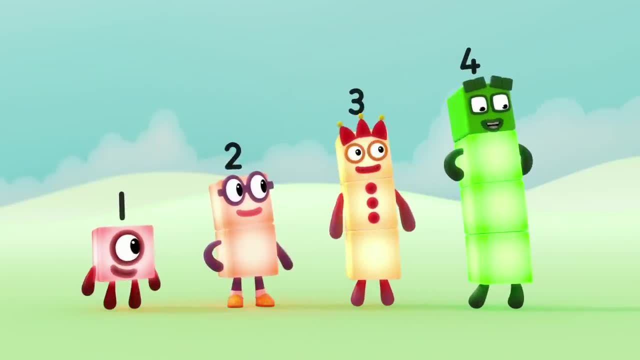 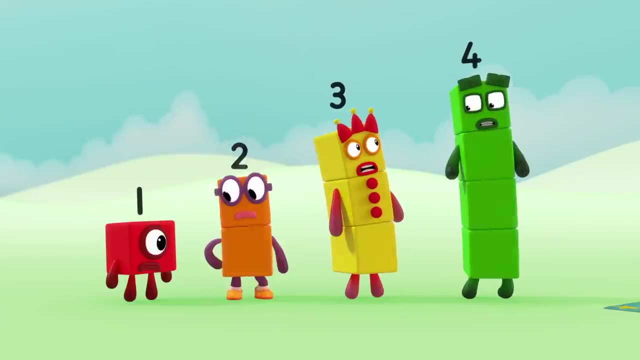 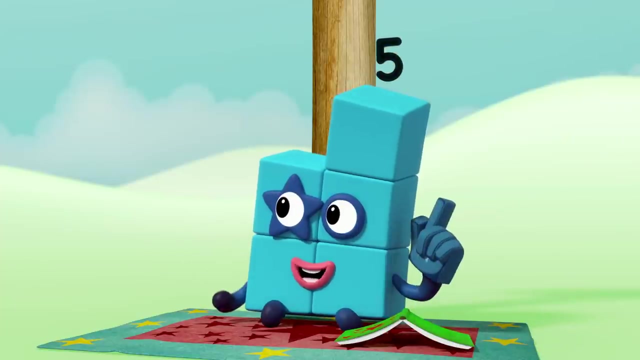 Hello, We're playing hide and seek, Want to join in. I would absolutely love to You hide and I'll seek. You won't find us sat there, Oh, will I not? now I'm good at this game. I'll find you and point you out. 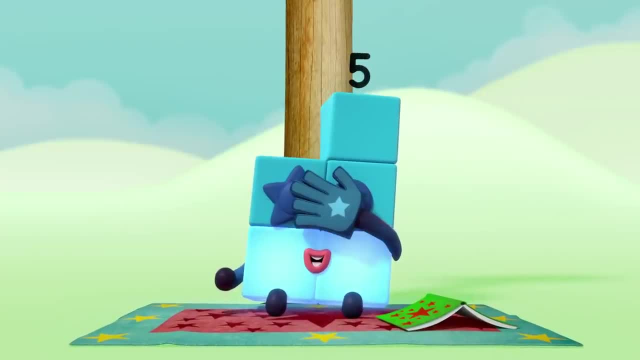 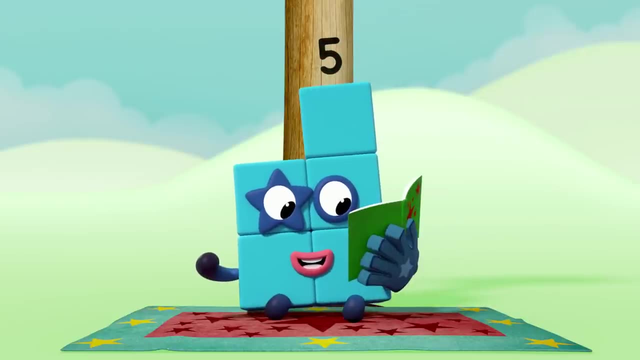 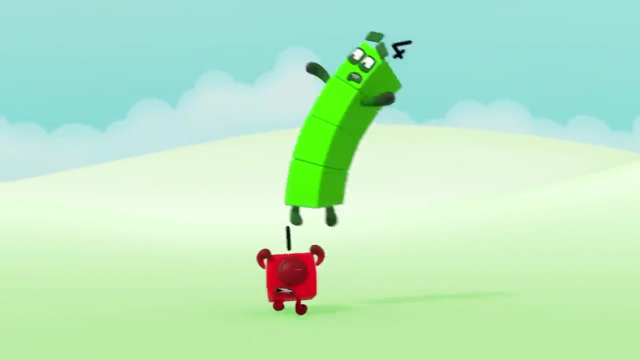 One, two, three, four, five. One, two, three, four, five. Ready or not? here I Get on with my book. Hey, hide behind me. Where can I hide? I know behind you Four. 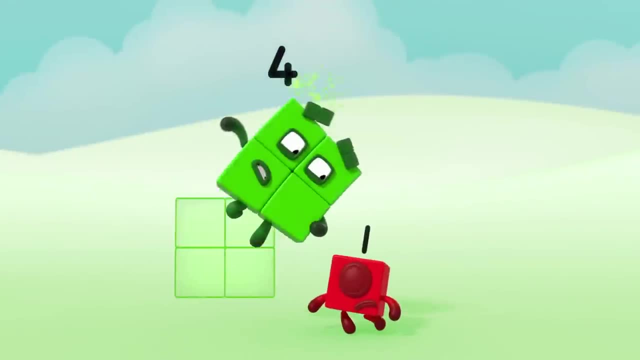 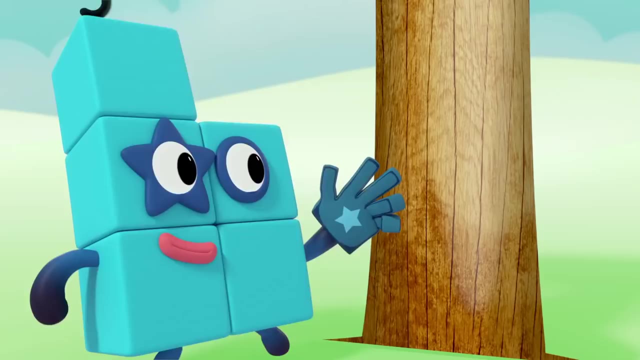 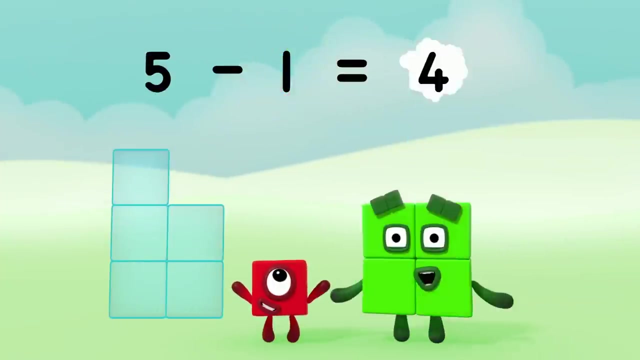 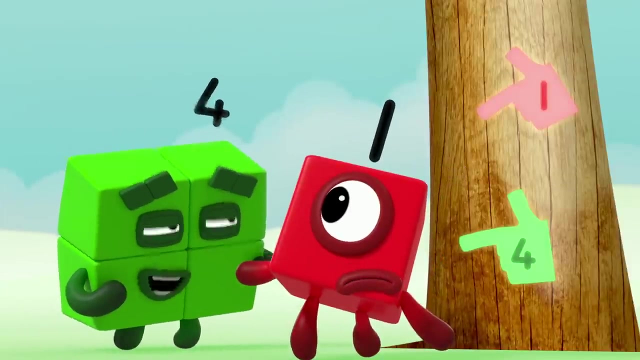 Huh, Oops, Huh. Four Plus one Equals Five. Ready or not, here I come. Find you four, find you one. Five minus one Equals four. Look, five, said she'd point us out. Five was right here. 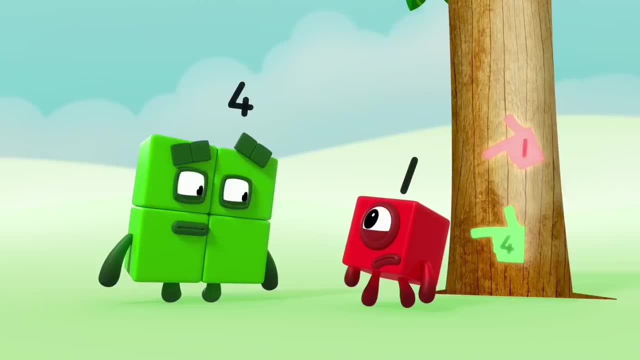 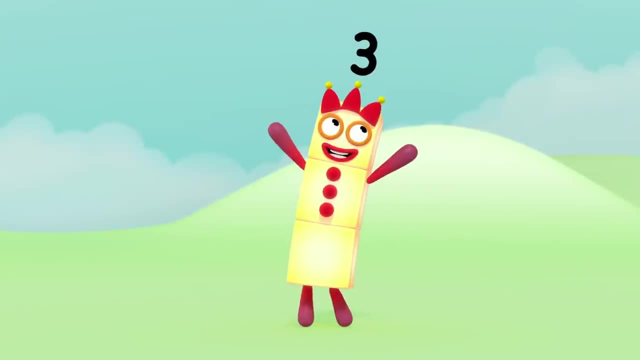 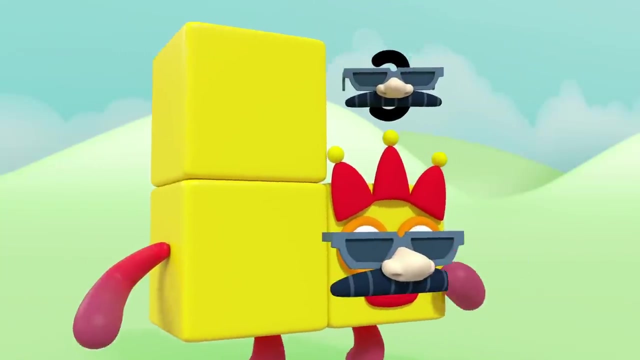 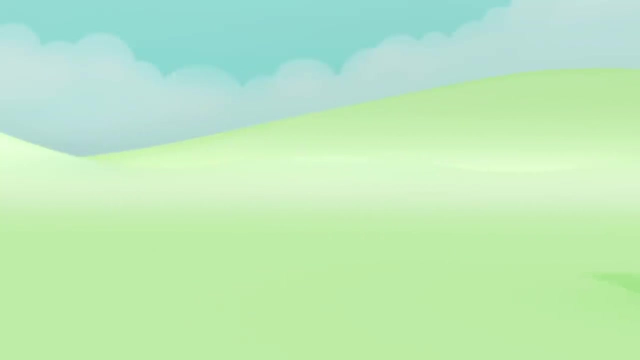 How, Hm, Hmm, hmm, hmm, I am three Master of disguise. Huh, huh, huh, ah, Shhh, Shhh. Two Plus three Equals five. Ready or not? Five minus three equals two. 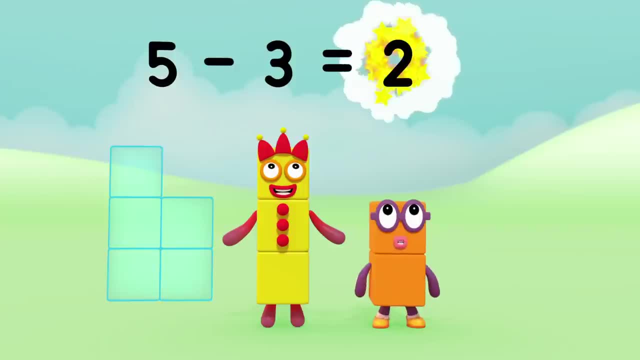 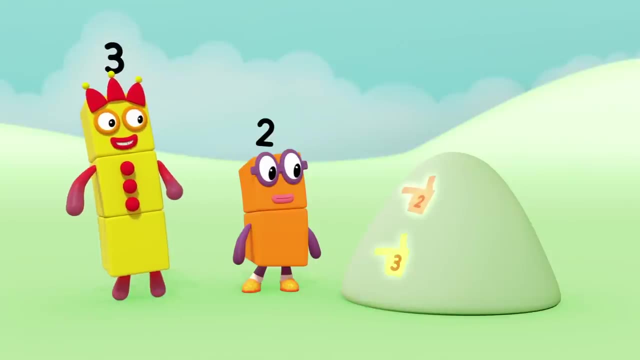 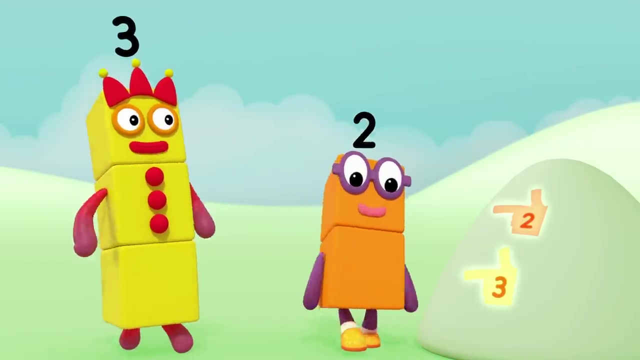 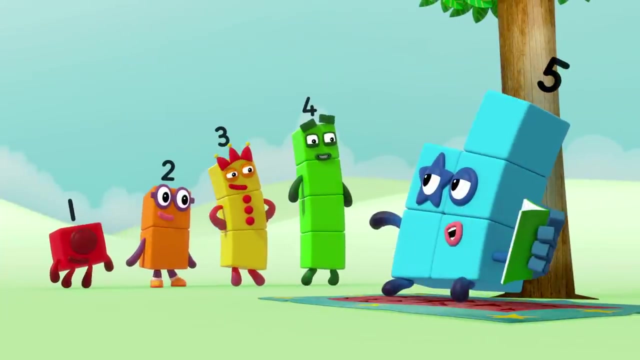 A pair of pointing prints. Five found us. But but how Uh Five You're here. How did you find us? I found you, I found you. How did you told you I was good? 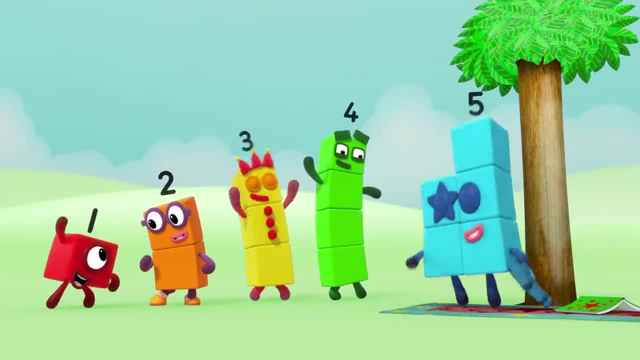 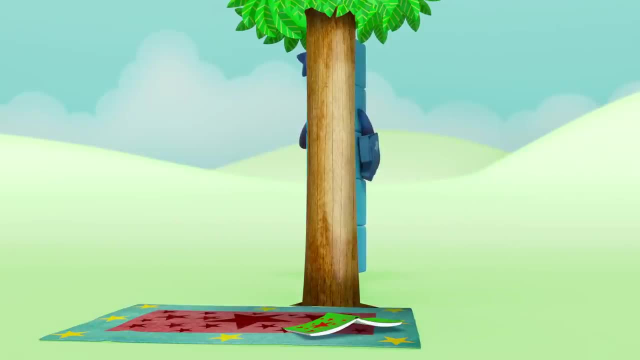 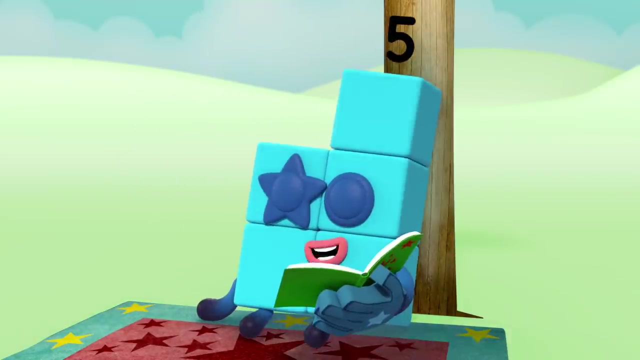 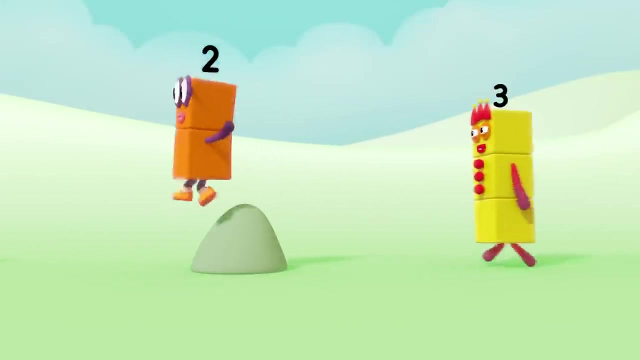 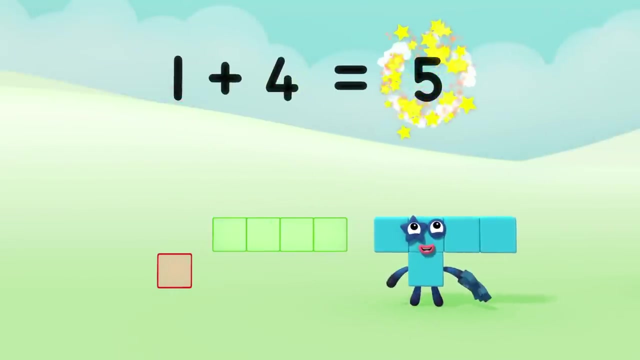 Now my turn to hide. Only day One, two, three, four. Ready or not? five here we come, Rock. One plus four equals five. Found you Amazing? Can you find me again? Five: 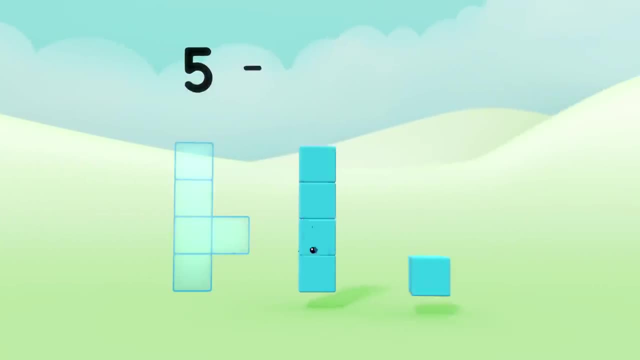 minus four equals one. Come on, Rock Rock Rock, Rock Rock. One, two, three plus two equals five. Found you Fine, Fantastic, Can you find me again? Five? 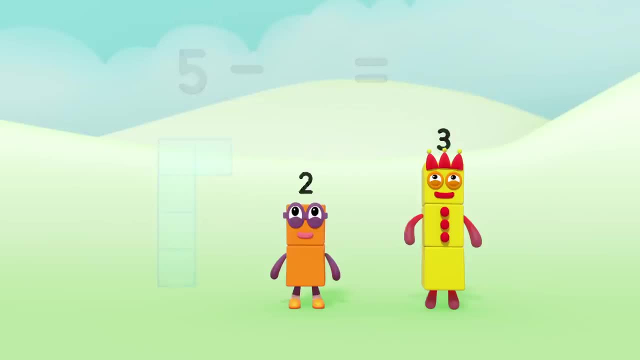 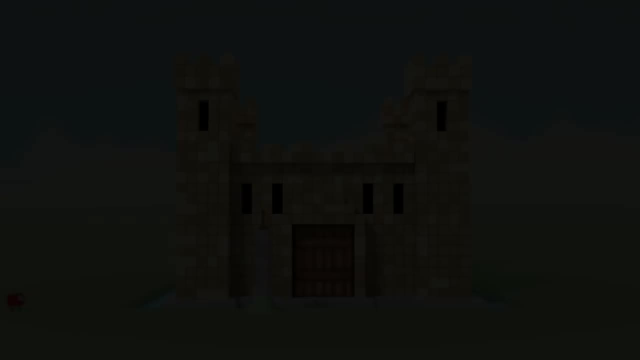 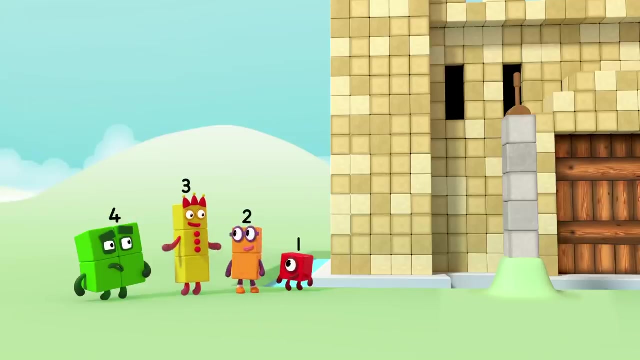 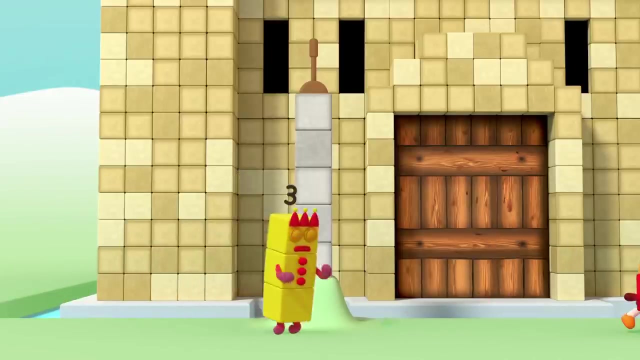 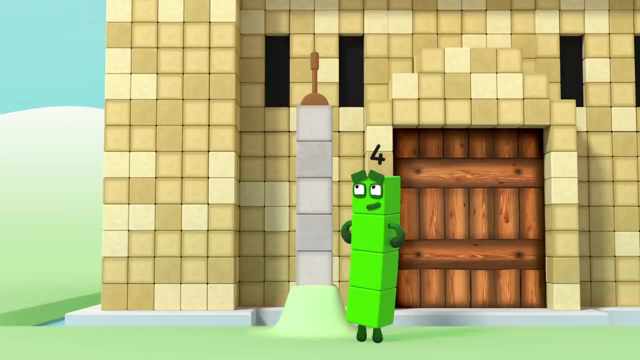 minus two equals three. Found you? Ha-ha-ha, Ha-ha-ha. Great, Maybe if we pull that handle. Oh, If only I was a little bit taller. Five's taller than four. So how do we get five? 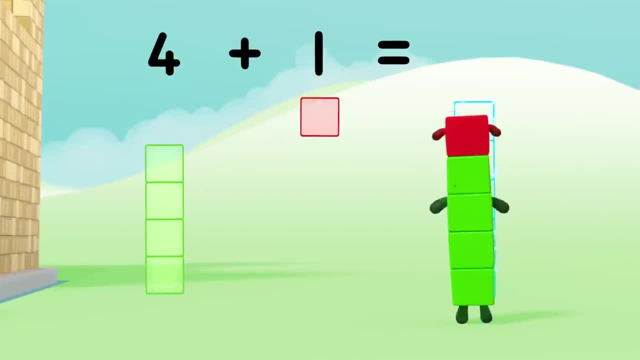 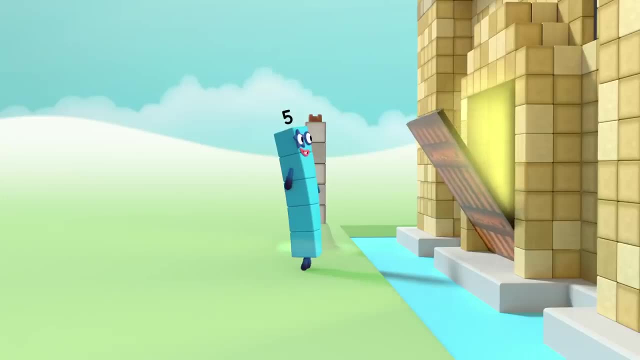 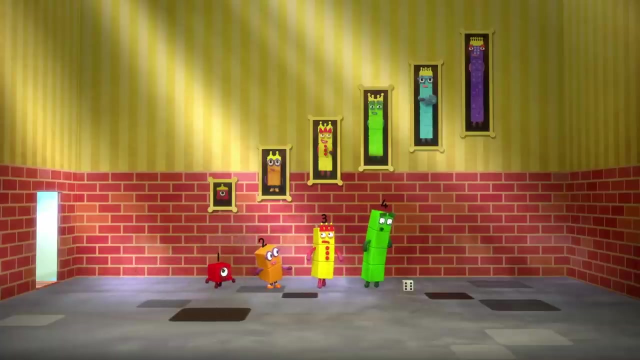 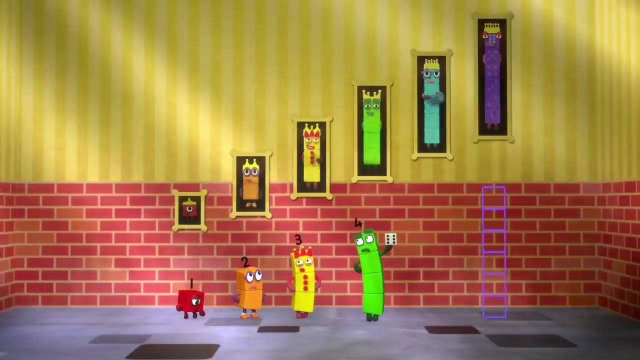 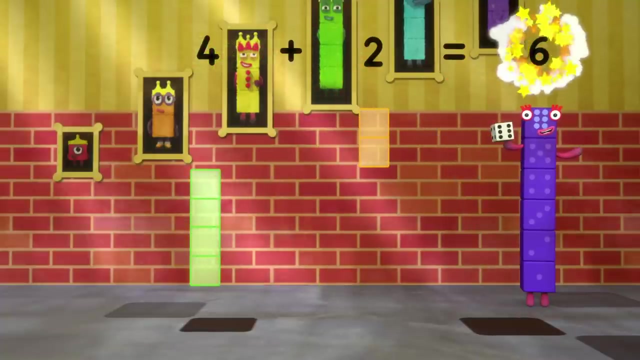 Four plus one equals five. Dead end. Six is good with dice. How do we get six? Four plus two equals six. Hello friends, Here's my advice. It's time for me to roll the dice. 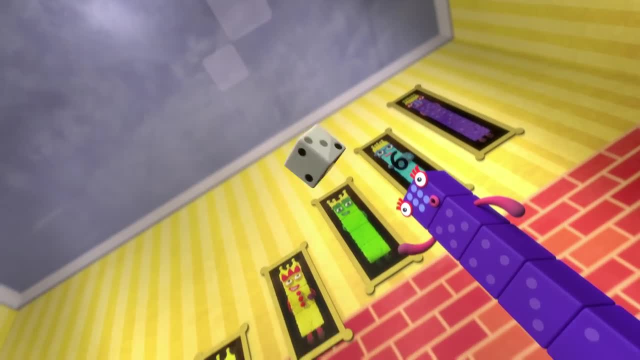 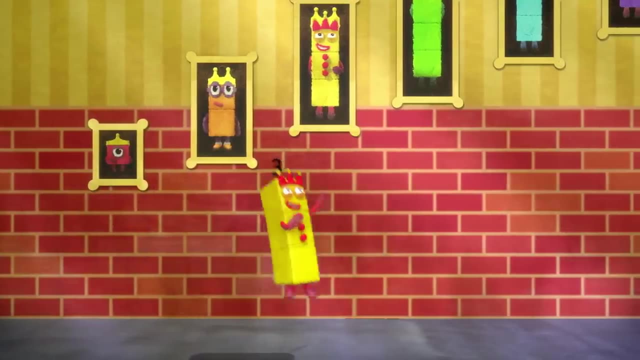 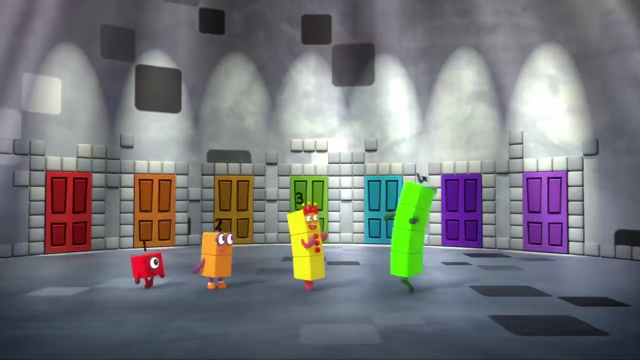 Watch me give a little throw and you'll know which way to go. One, two, three, One two, three. Follow me. Seven doors. Which door is right? Maybe seven? You can help. How do we get seven? 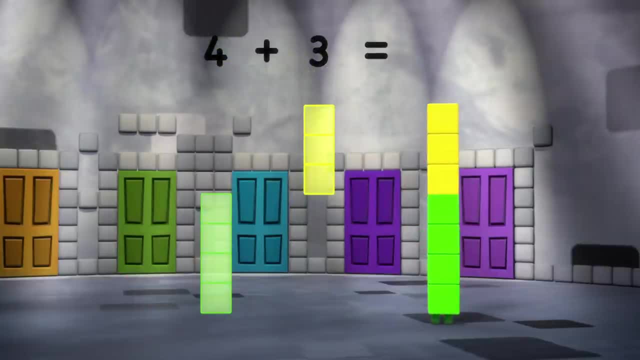 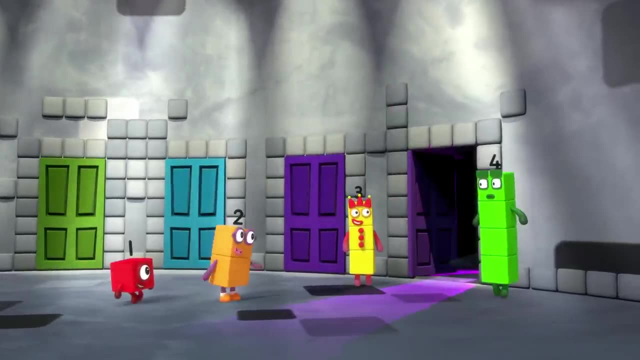 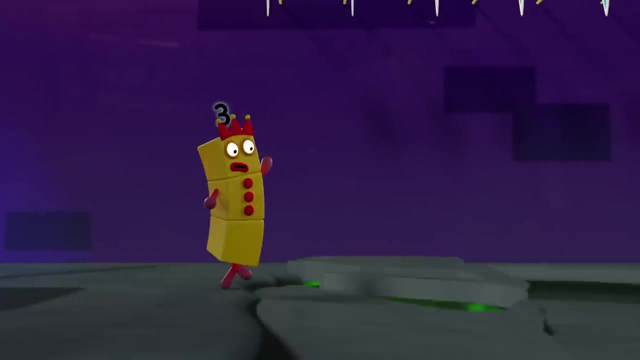 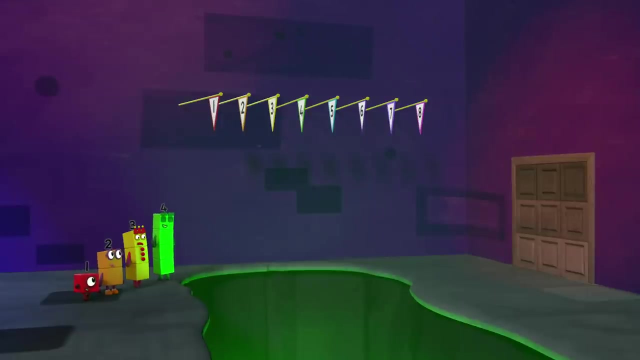 Four plus three equals seven. Oh, I feel lucky This way. Easy-peasy, Look amazing, We're stuck. No, we're not. We could swing from the flag poles. We'd need someone with very long arms to stretch that high. 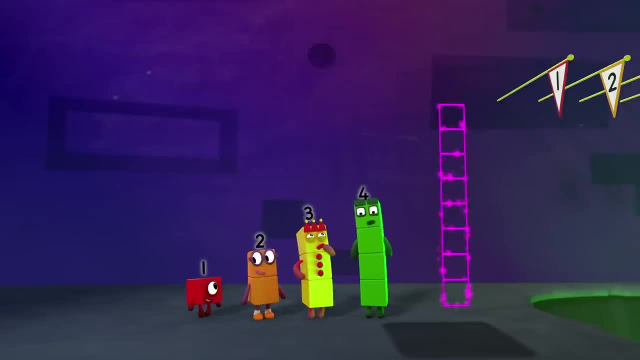 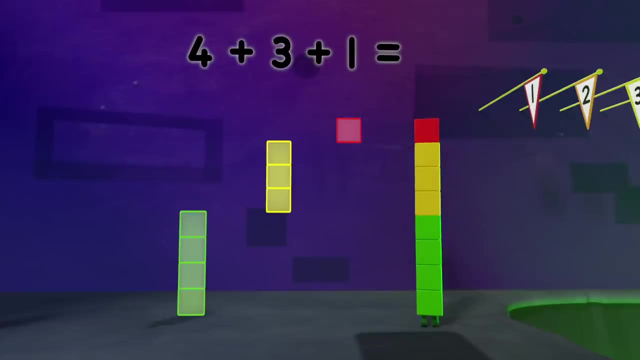 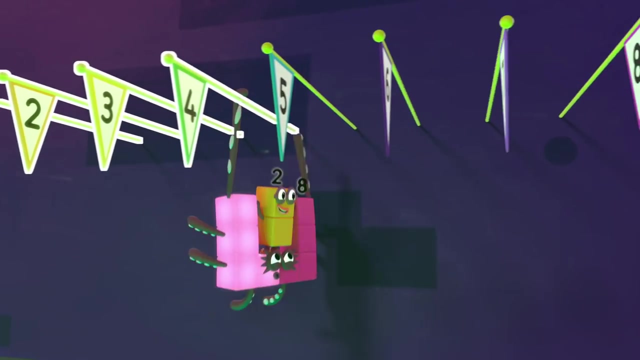 Eight, How do we get eight? Four plus three plus one equals eight. Octoblock swing One, two, three, four, five, six, seven, eight Swing. Oh, we're stuck. 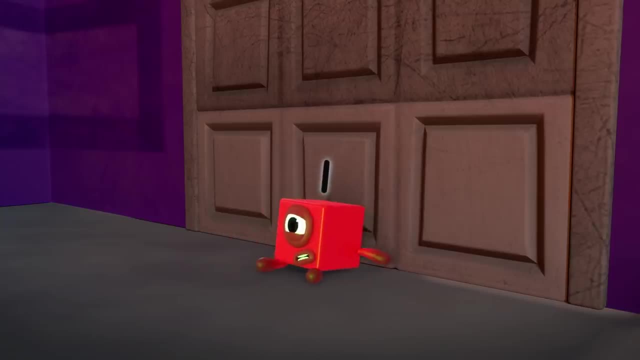 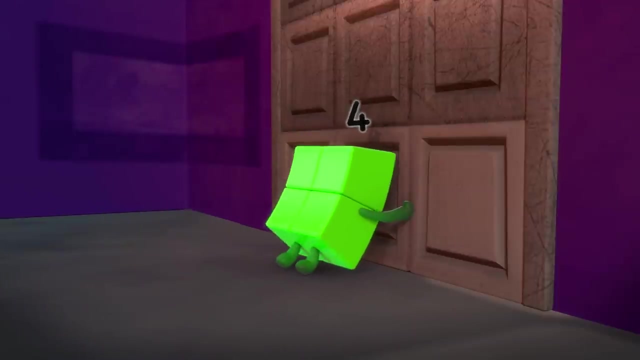 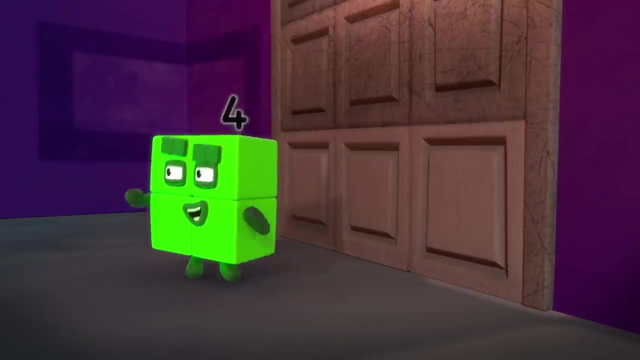 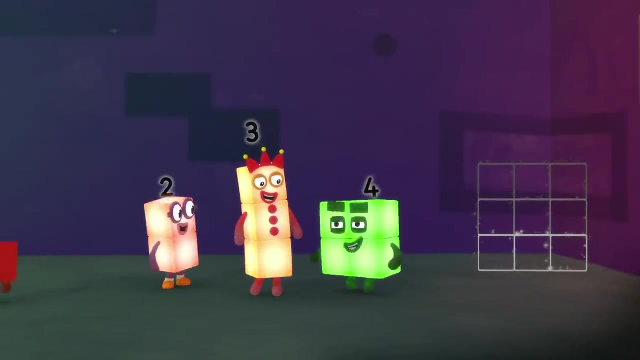 That was close. Listen, Oh look, It's stuck. The squares are strong. Let me try. Oh, oh, Enough. now We need a bigger square. Nine: How do we get nine, Six plus nine quickly? 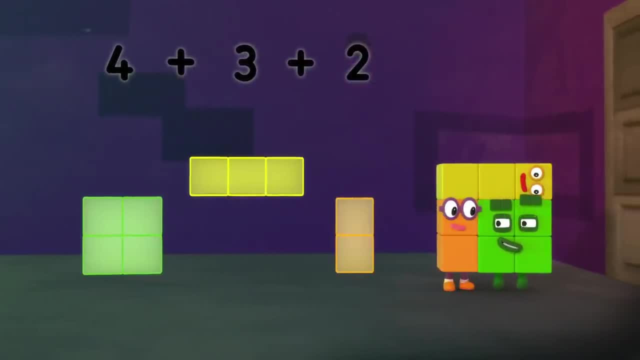 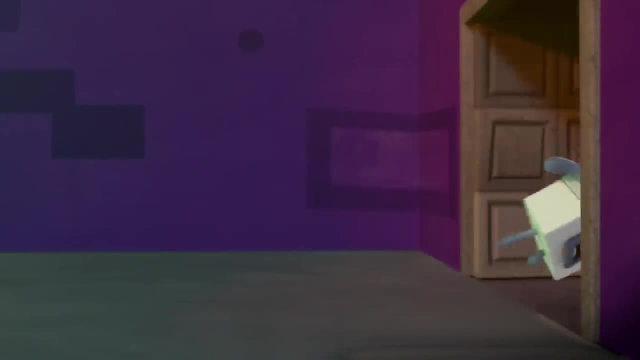 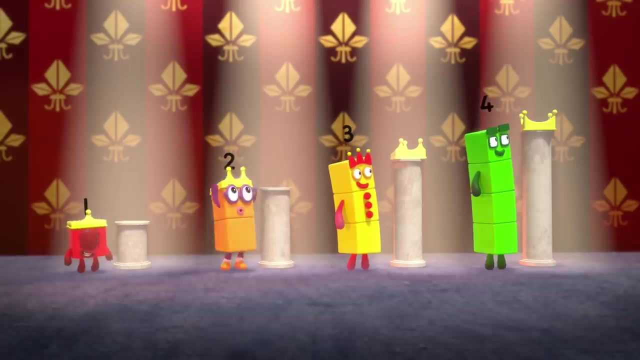 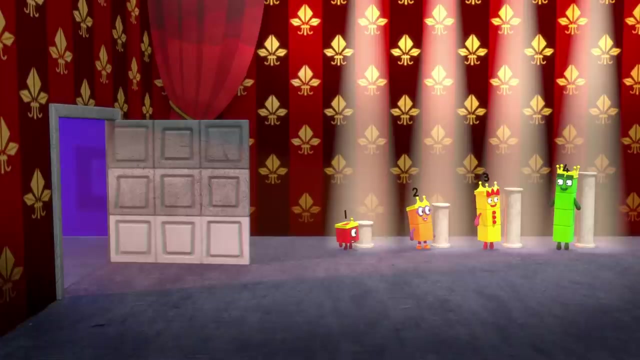 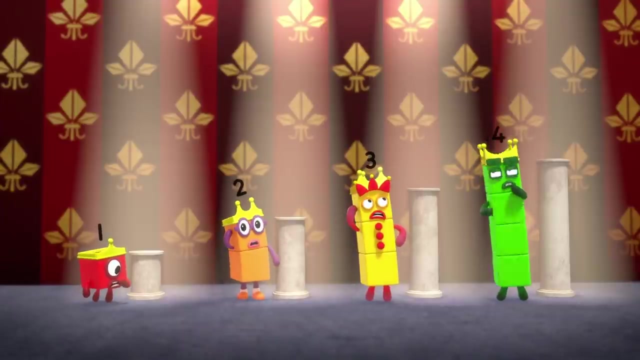 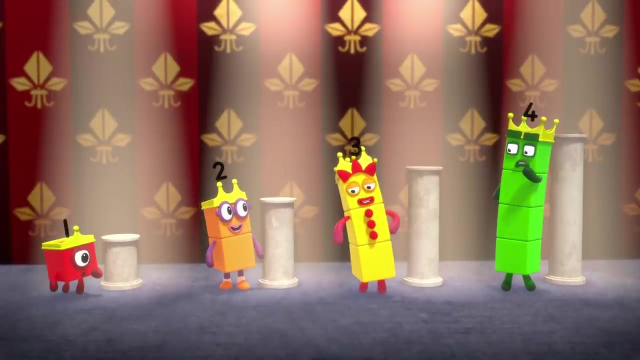 Four Plus three plus two equals nine. Thanks, One, two, three, four, Four crowns. Uh-oh, How are we going to get out? Uh-oh, If ten was here, we could rocket out through there. 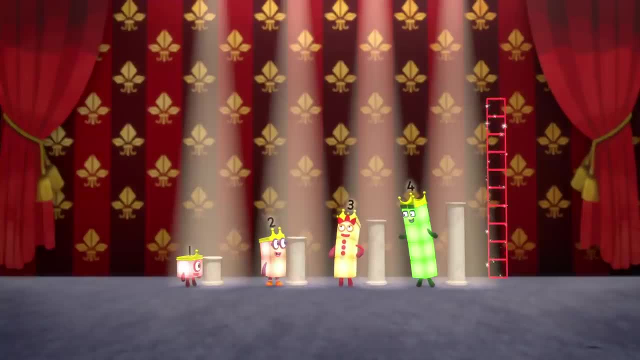 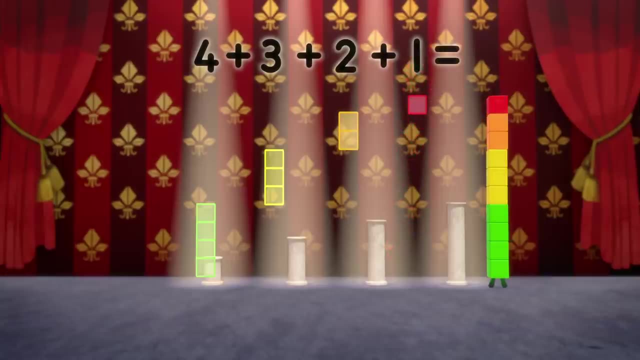 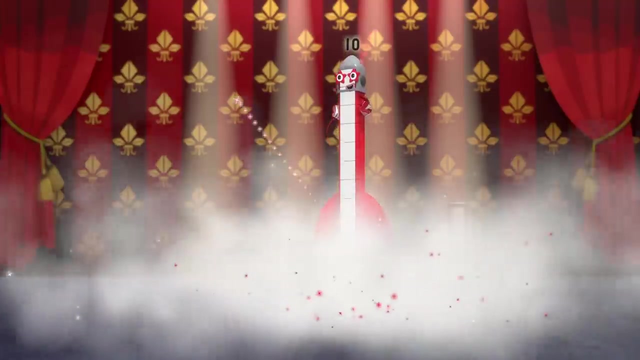 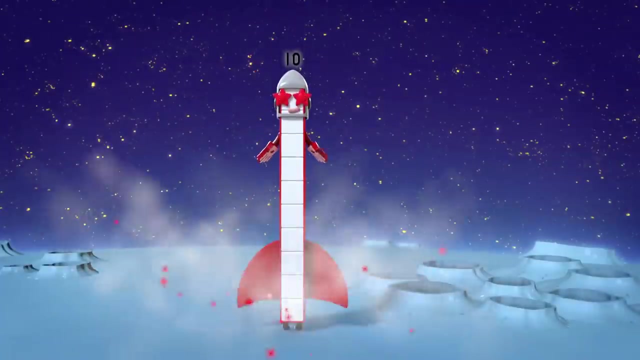 How do we make ten All together? now? Four plus three plus two plus one equals ten, Ten, nine, eight, seven, six, five, four, three, two, one. Blast off Number ten up on the moon, and my friends will be here soon. 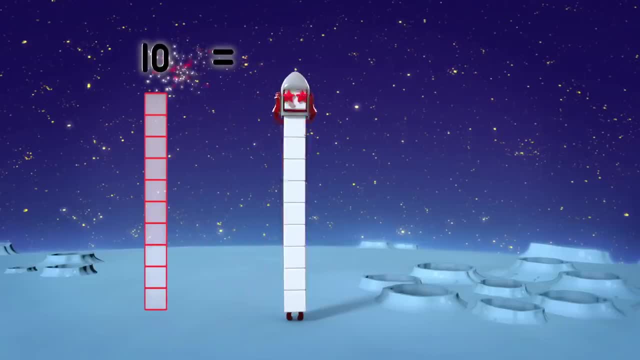 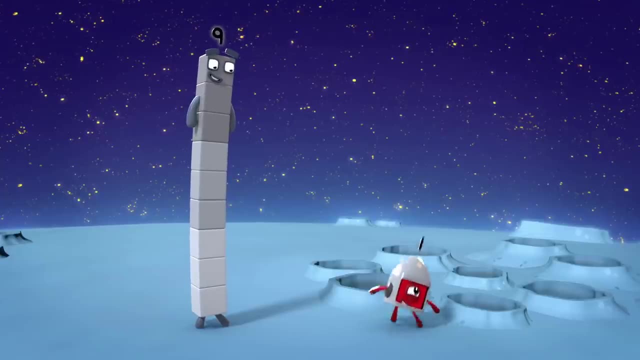 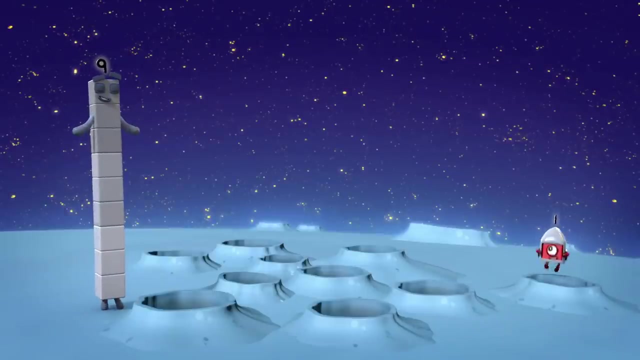 Ten equals nine plus one. One small step for a number, One giant hop for number kind. We're on the moon, Not on the moon. We're on the moon One, two, three, four, five, six, seven, eight, nine. 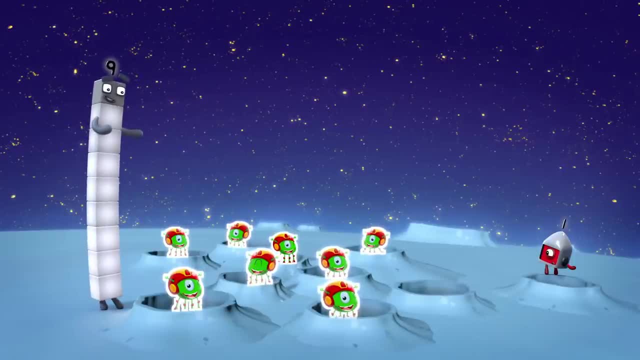 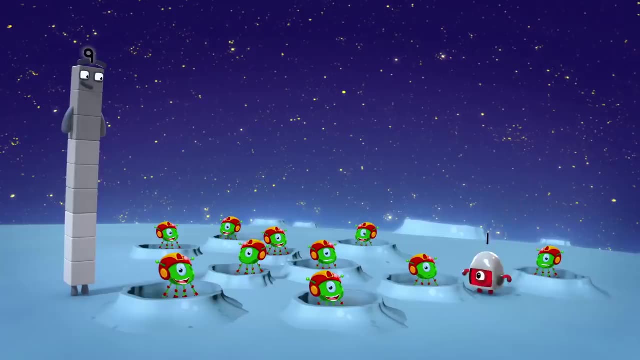 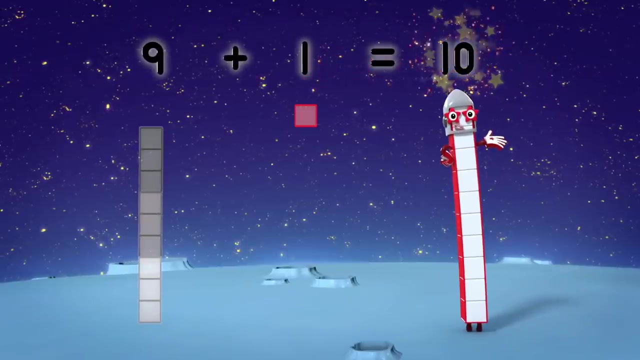 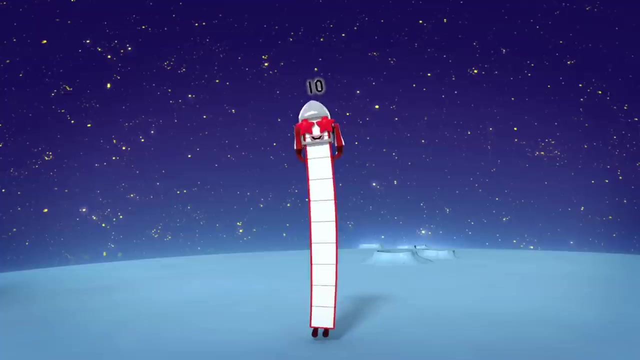 Nine aliens And one more is ten. Nine plus one equals ten. Number ten back on the moon. Two more friends will be here soon: Ten One Two One. Ten Ten equals Eight plus two. We're on the moon. 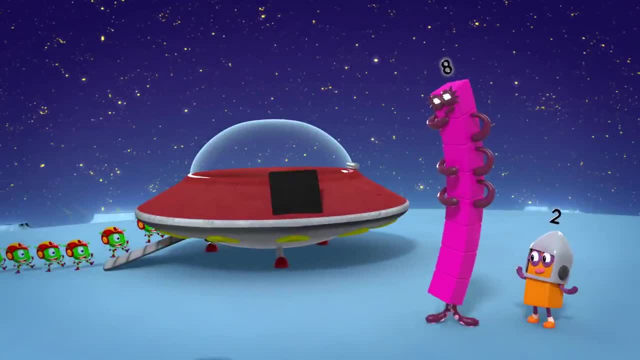 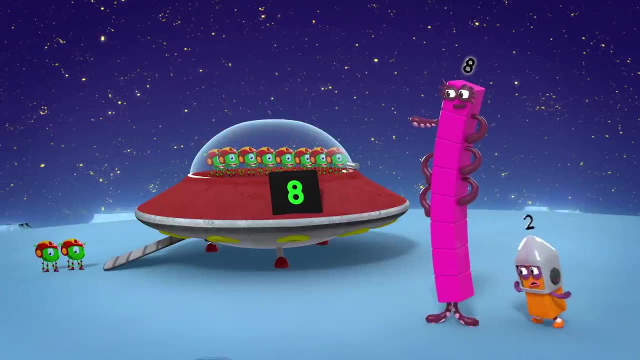 Eight And two. How did we get here? Haven't a clue? One, two, three, four, five, six, seven, eight, Eight aliens all heading home. Oh no, There's no room for those two. 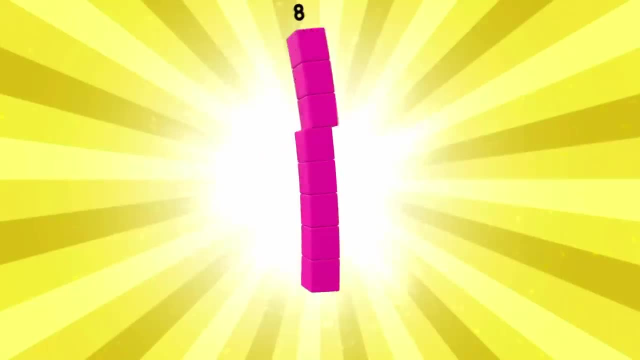 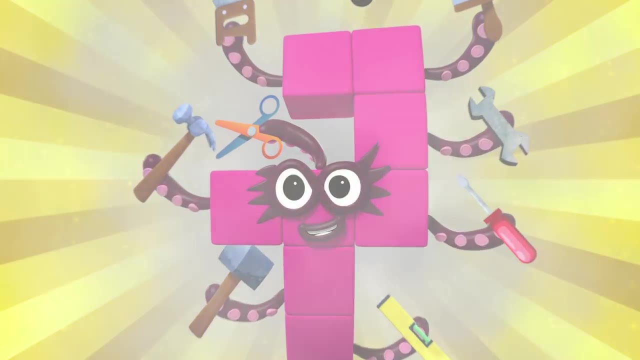 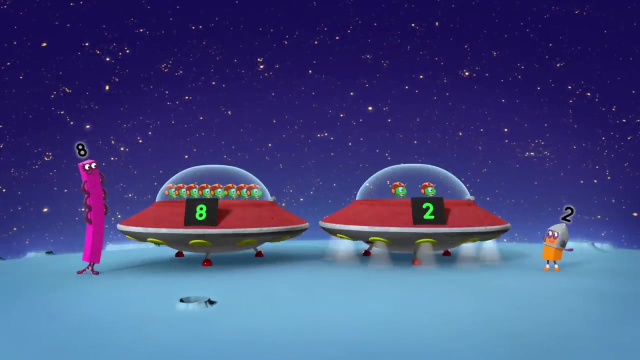 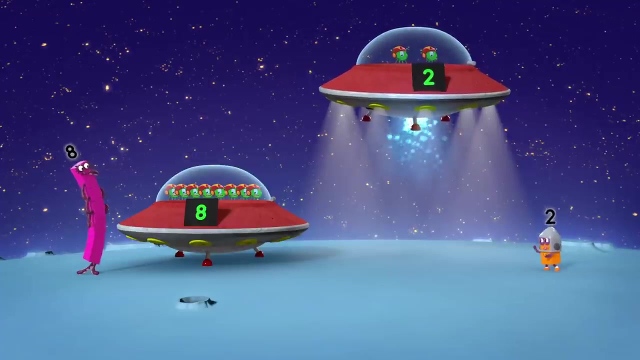 Never fear, Octoblock is here. Octoblock: Bill One, two, three, four, five, six, seven, eight, Eight. Bill Two: flying saucers, Good work. Ah, Oh, come back, It's not starting. 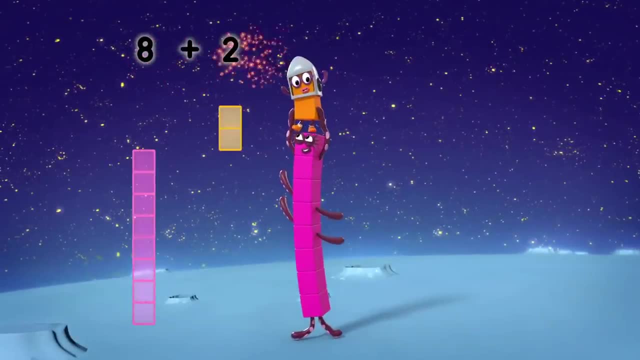 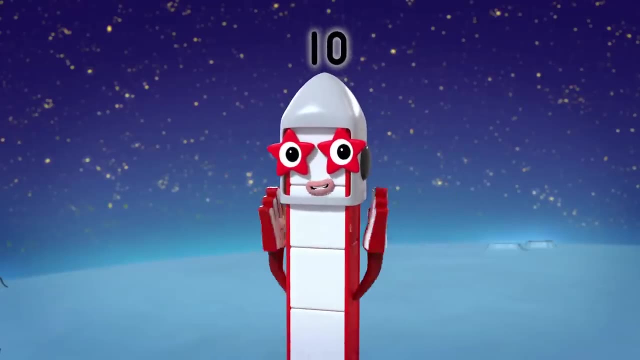 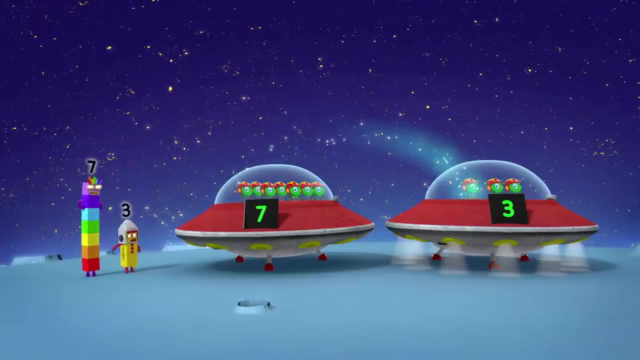